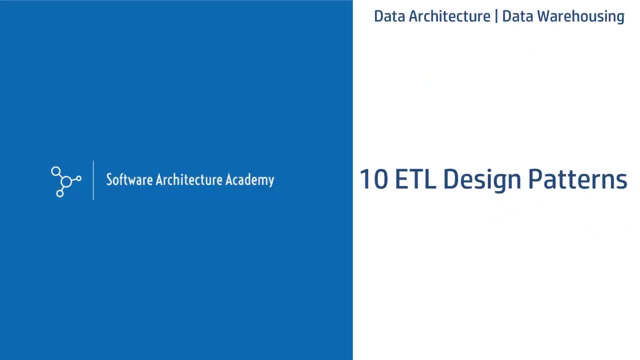 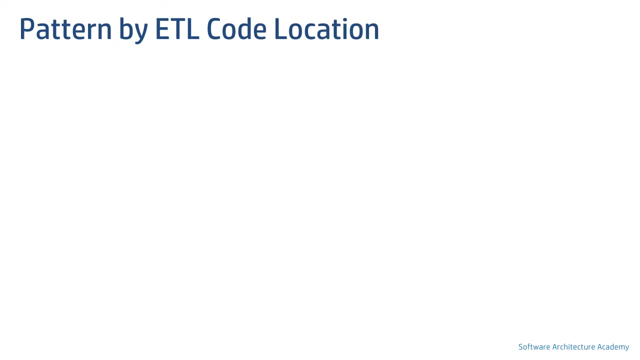 Hi everyone. today we will walk through 10 different ETL design patterns. This video is part of data warehousing series. Knowledge of ETL patterns is must in order to build a data warehouse, So let's get started. So first, segmentation of patterns is by where exactly the ETL code or processes are located. 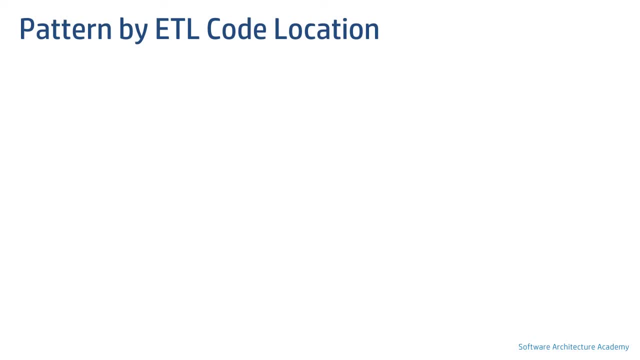 We will keep it simple, since this is a design pattern. Consider a source system and a target data warehouse. ETL code can reside in the source system, where it usually pushes the data to its destination. This is our very first pattern: ETL code at source system. 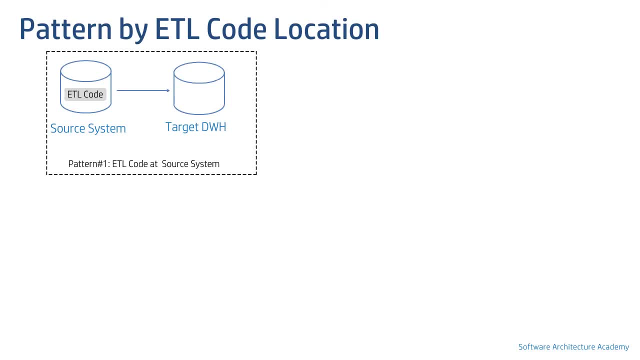 Likewise, our next pattern is where the ETL code resides in the destination or target data warehouse. We will keep it simple, since this is a design pattern. Consider a source system. A pull mechanism is usually a pattern of the destination or target data warehouse. 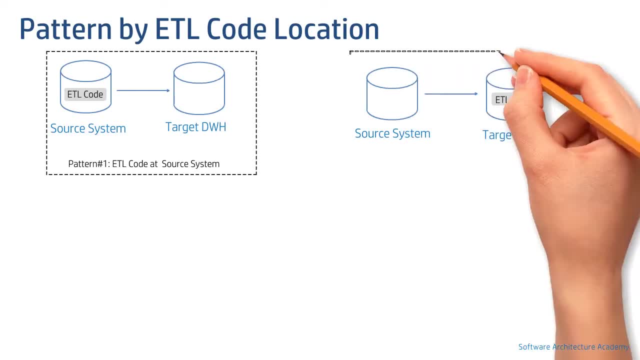 used by the data warehouse to connect to the source system and obtain data. usually, a database connection is established by the ETL tool or package. our third pattern introduces another aspect, which is the ETL code residing on a dedicated ETL server. here the ETL server pulls. 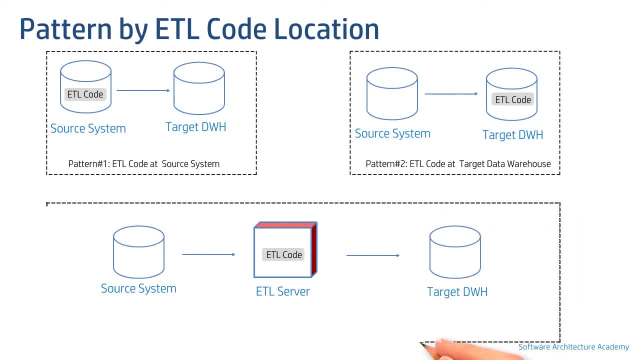 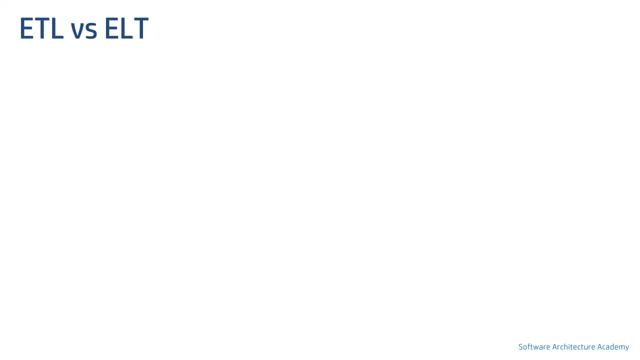 the data from source system and pushes it to the target data warehouse. so these were our first three design patterns. next we will be three ETL versus e LTE patterns. these are based on where the transformation is exactly performed. I will be discussing two patterns in this very diagram. 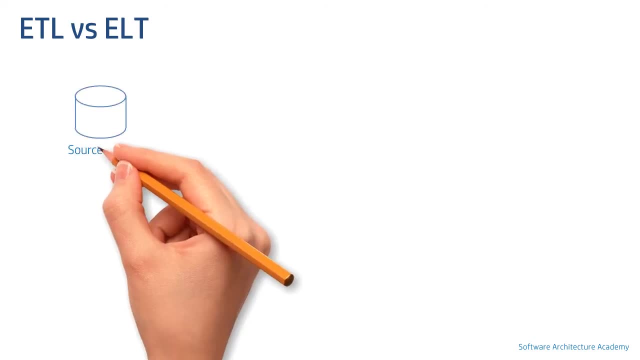 together. consider a source system in ETL server and a target data warehouse from a frigided database. if a data warehouse is a sub 85 or ability to handle parameters such as I, will be resulting there as so: a source system for a data warehouse for a target data warehouse. 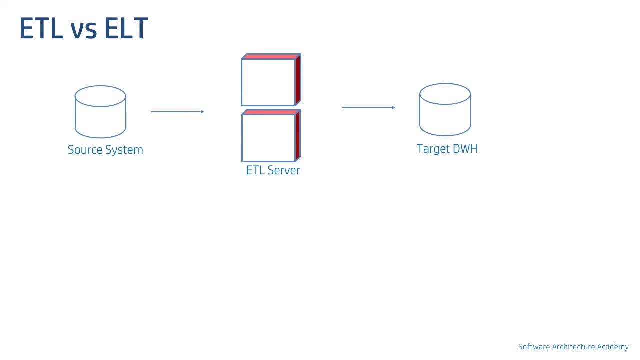 our previous diagram. ETL server extracts data from a source system, performs transformations and then loads it into the target data warehouse. This is ETL pattern. Two variants of this can be whether the transformation is performed in a dedicated stage on disk, or if it is performed. 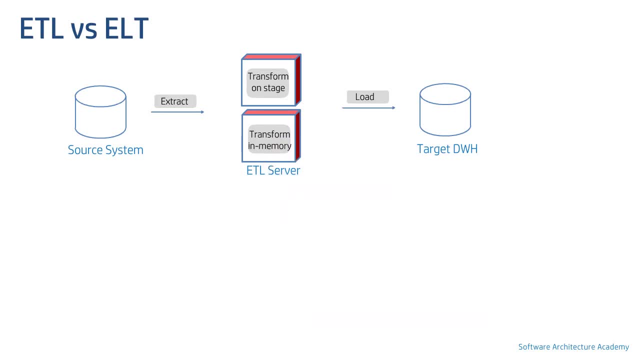 in memory of the ETL server. So those were our pattern 4 and pattern 5.. Now let's talk about ELT. As the sequence in ELT suggests, the data is first loaded into the data warehouse and transformations is then performed. ELT is best used when the data is enormous. That 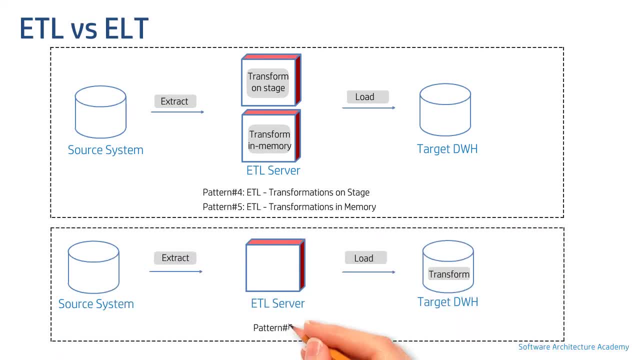 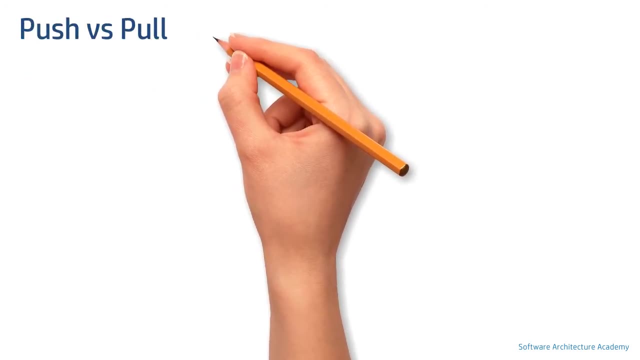 was our pattern number 6.. We will talk about something that we touched base upon earlier, but now in detail, which is 4: push versus pull patterns. Let's discuss both push patterns together. Consider a source system that sends data either directly to a target data warehouse or directly to the. 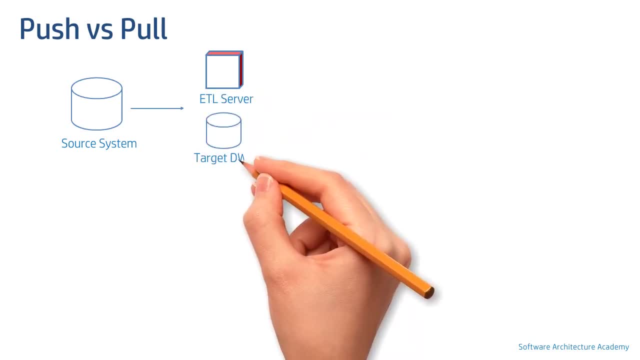 target data warehouse. This is a system that sends data either directly to a target data warehouse or directly to a target data warehouse. This is a system that sends data either directly to a target data warehouse or directly to a target data warehouse, or via a dedicated. 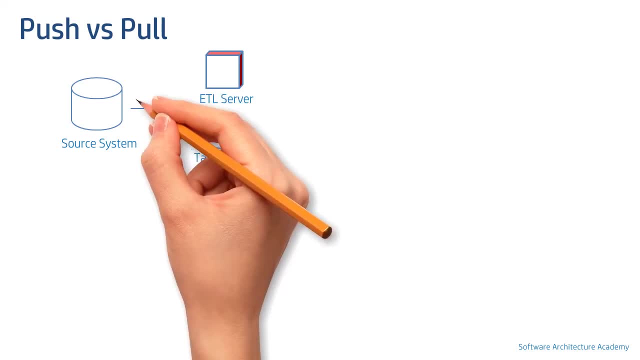 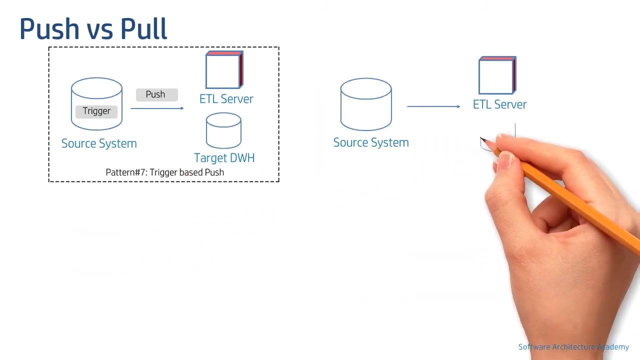 ETL server, Push is initiated at the source system. It can be initiated via a database trigger, which is our pattern number 7. Or it can be scheduled via a job, which would be our pattern number 8.. A pull is initiated from ETL server or a target data warehouse. 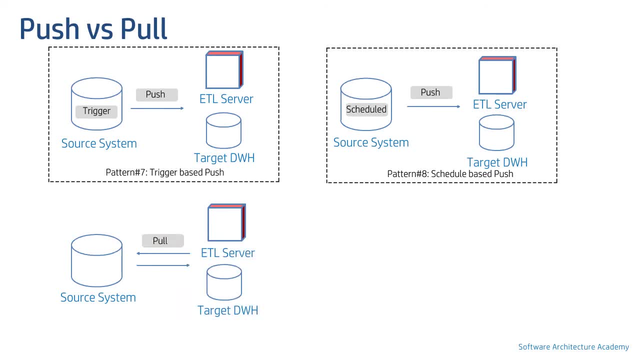 Broadly. it can be initiated by two means: First, scheduled, as per example before, and second, based on log file tailing. In this pattern, a process tails a log file located on a source system and looks for specific actions or keywords. 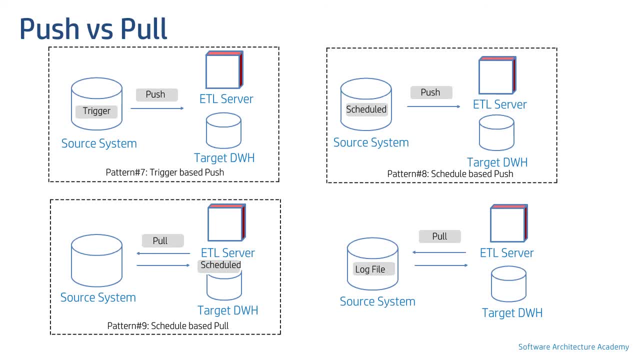 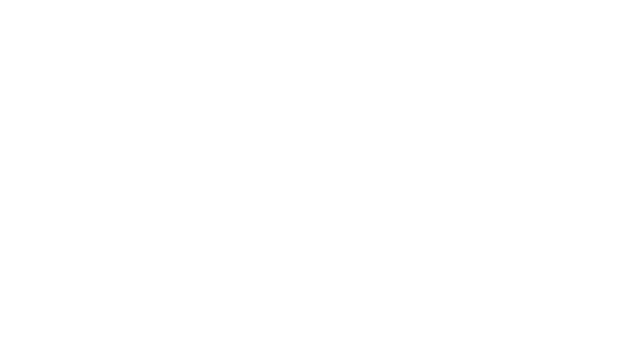 When those actions or keywords are encountered, a data pull is then initiated. These would be our final patterns, pattern 9 and 10.. So that's all we have for today. If you like this video and had a good learning experience, then do check out our other videos. 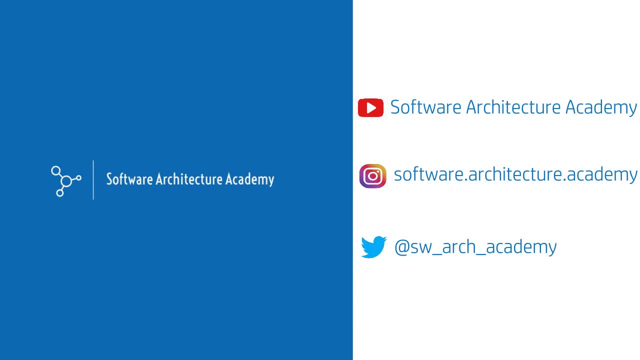 Do like and share. Also, subscribe the channel for latest videos and trends in the world of architecture. See you in the next video. Transcription by CastingWords.